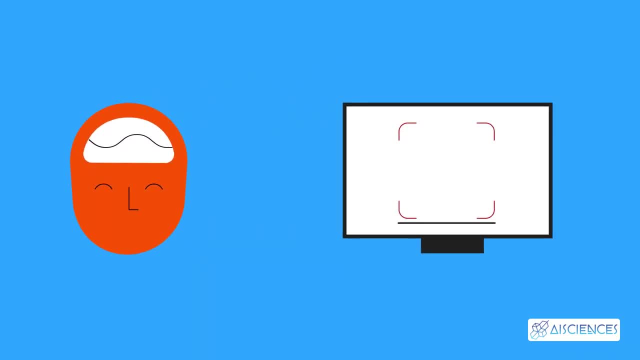 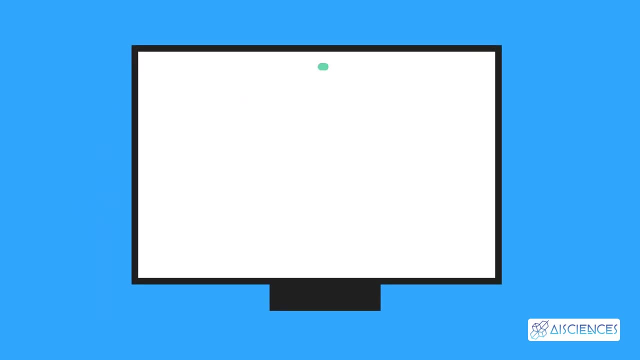 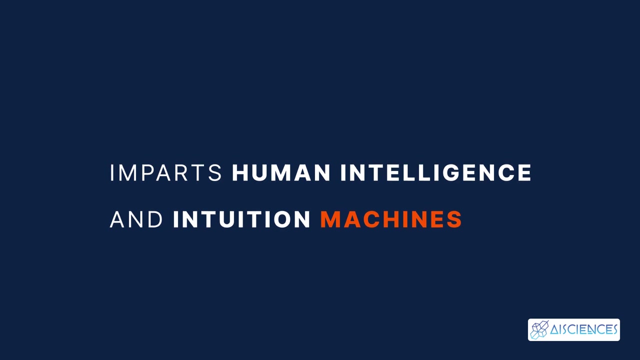 the complex human visual system. This field enables computers to identify objects in images and videos and process these objects in the same way that humans do. The computers then provide appropriate output. So, in simple terms, computer vision imparts human intelligence and intuition to machines. In this short video I'm going to discuss 5 real-world applications of computer. 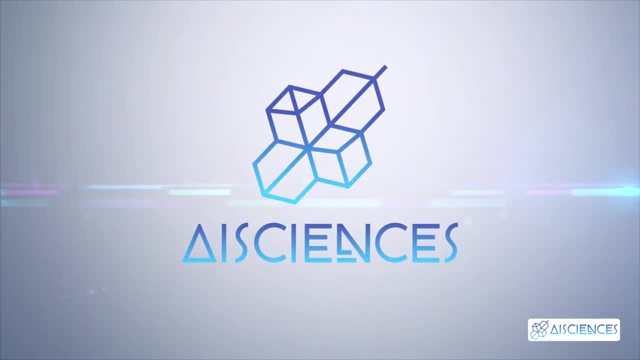 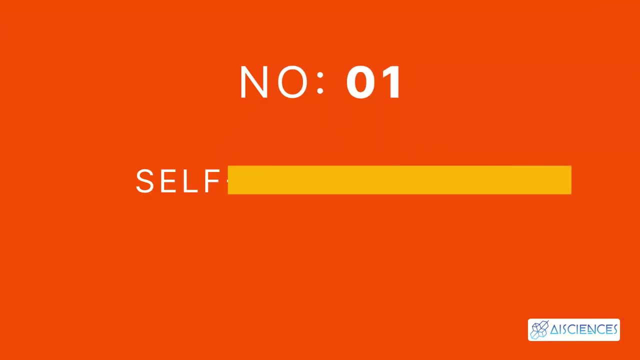 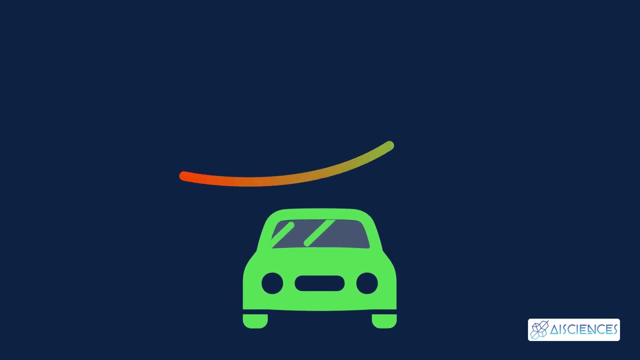 vision. 1. Self-Driving Cars. Experiments on self-driving cars have been conducted for close to 100 years now, But thanks to rapid advancements in computer vision in the last 10 years, computer vision has become more and more popular. In the last 10 years. many major automotive manufacturers are testing driverless car systems. 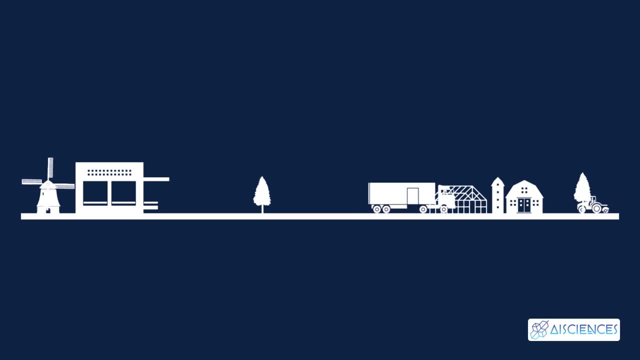 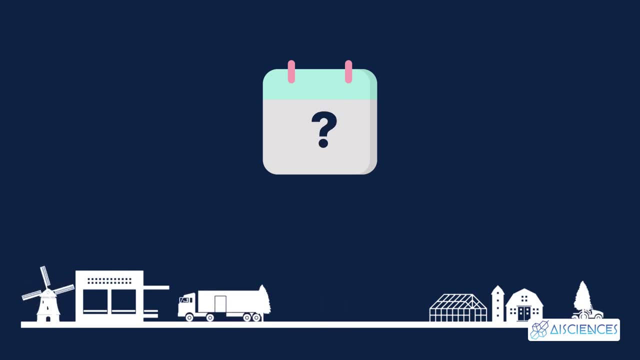 Driverless cars are soon expected to change the way people get around in a big way. The exact timeline as to when driverless cars will be widely available is not yet clear, though, But one thing is certain: Fully autonomous vehicles will soon be a reality. Autonomous. 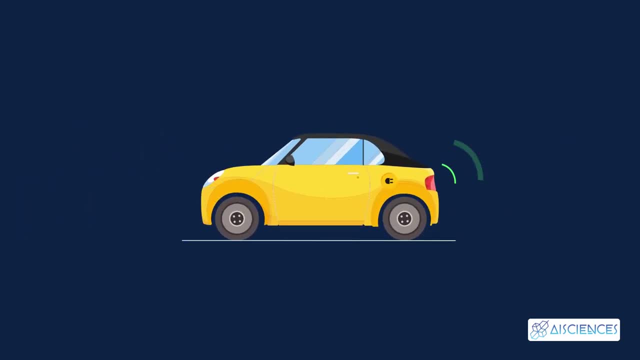 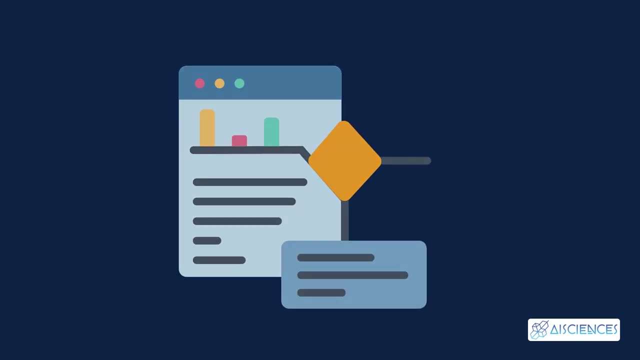 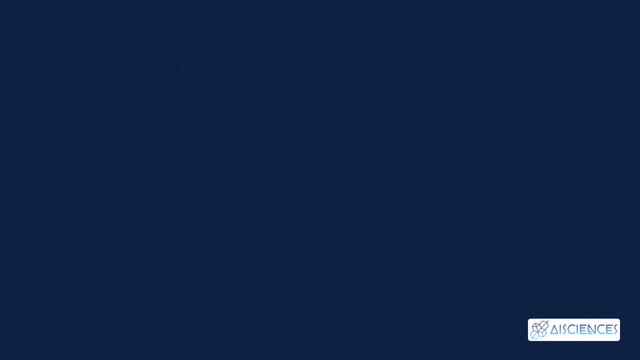 cars track the surrounding objects with cameras. Then, based on the inputs received, the cars react according to what's happening in their driving environments. Advanced algorithms in autonomous vehicles control path planning, driving scene perception, motion control and distance judgment. The top benefits of autonomous cars to humanity will include: 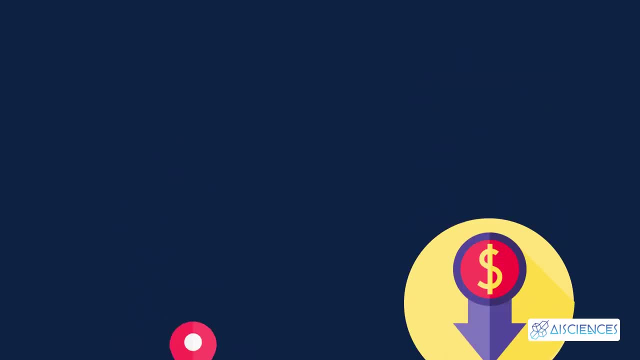 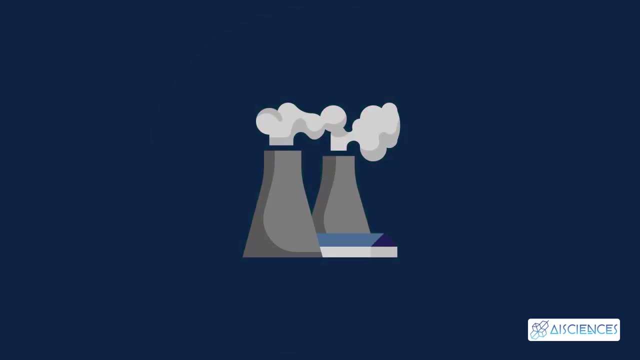 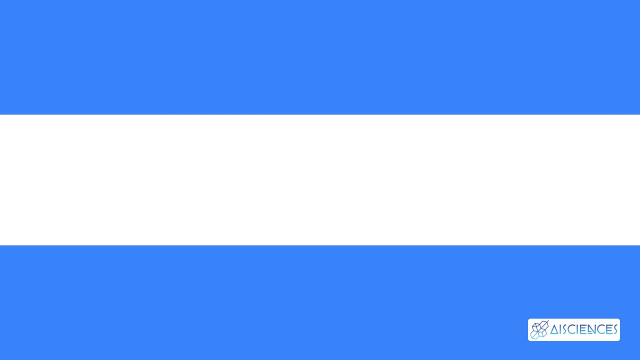 safer roads and lower transportation costs. Also, the air pollution levels in cities will fall drastically. The use of fewer fossil fuels will result in a massive drop in the emission of greenhouse gases. 2. Waste Management and Recycling. Advancements in computer vision that enable face recognition also power AI-based waste. 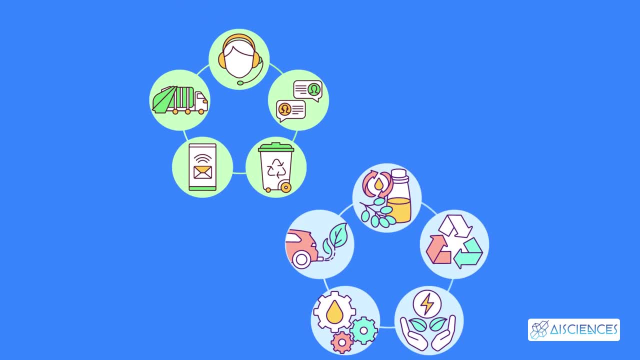 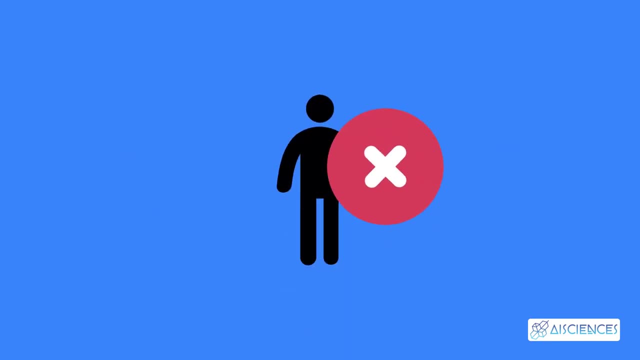 recognition technologies. The latest waste recognition systems identify, check and analyze waste composition at scale. Businesses no longer need to rely on human spot sampling to understand the real value of their material In waste management. computer vision is used to assist machines in sorting waste. Technological developments empower machines. 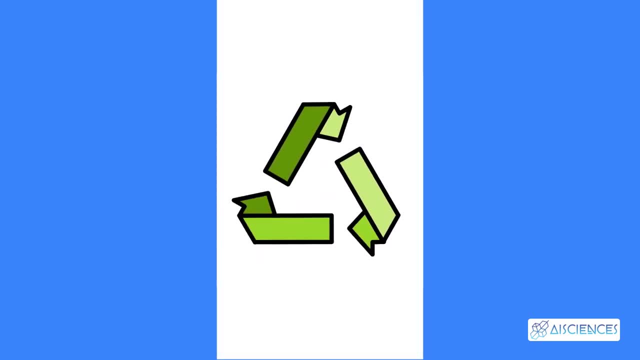 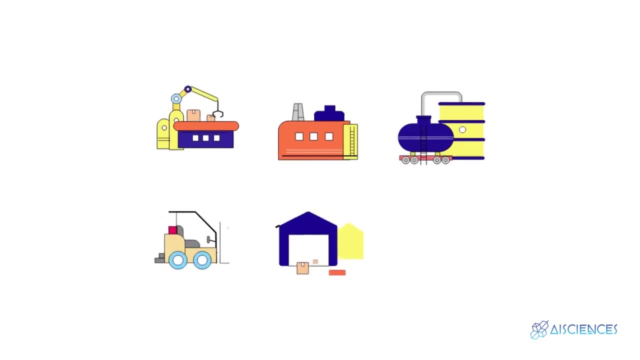 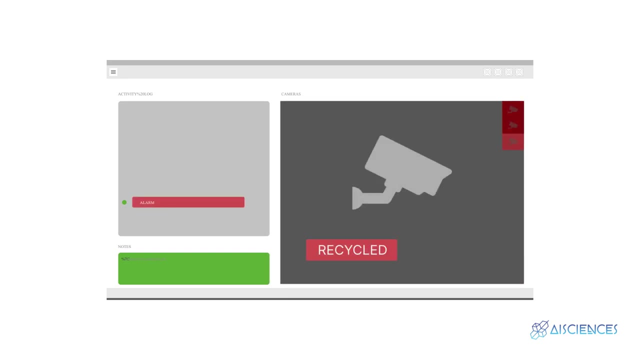 to sort waste in an increasingly human, or even better way. Many companies in the waste management and recycling sector apply this technology to reap the advantages of a reliable and efficient system. Waste monitoring via object detection can automatically sort waste bins, facilities and trucks. Smart bins can then accept recyclable materials or unwanted waste. 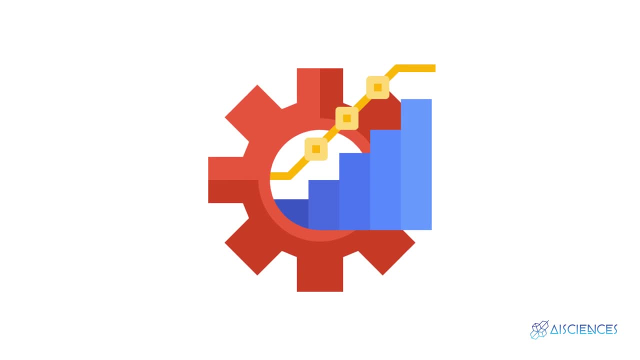 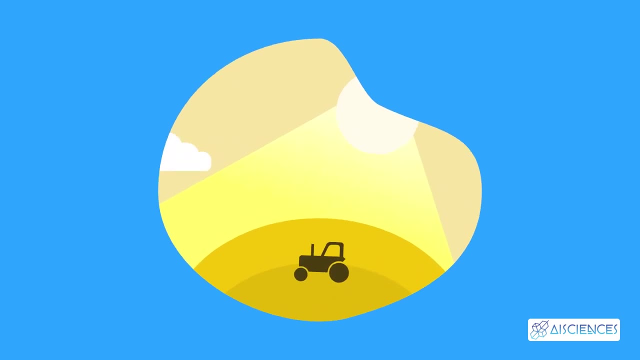 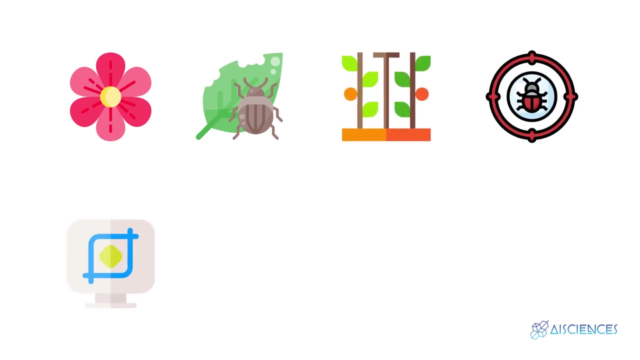 Hence, the entire waste management and recycling process can be easily optimized. 3. Agriculture: Computer vision is used to automate various activities in agriculture, such as flowering detection, plant disease detection, crop monitoring, insect detection, plantation monitoring, de-weeding, harvesting and agricultural product quality testing. Aerial imagery provided by 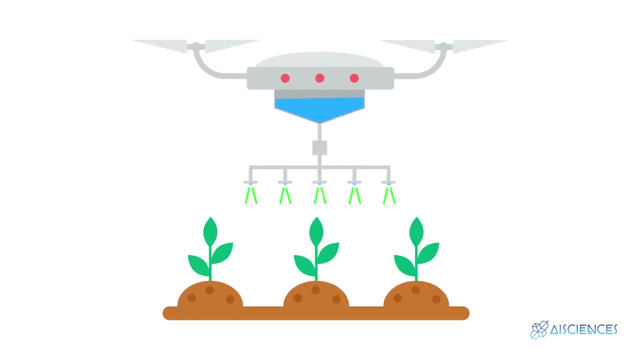 drones records detailed information about the condition of the soil and crop. Computer vision assists agriculture by increasing yields. Drones are a vital element in precision agriculture. They cover a significant distance and capture enormous amounts of data via a pre-installed camera. The camera is trained to detect adverse weather conditions. 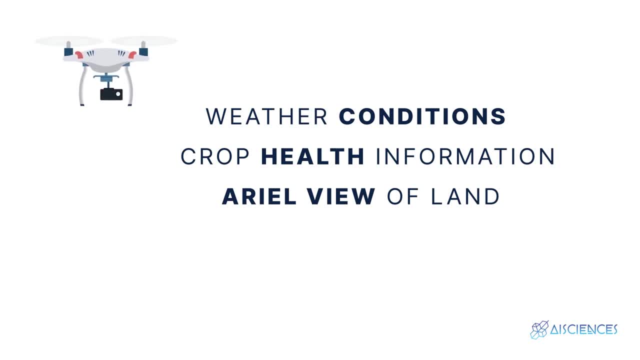 provide crop health information, present an aerial view of the entire agricultural land and identify soil conditions. The data collected from these drones and satellite images is fed into smart systems. These systems analyze large volumes of complex data and provide reports. These accurate reports enable farmers to adopt more efficient growing methods. 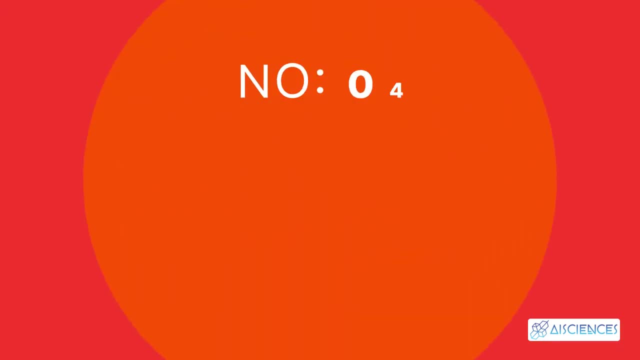 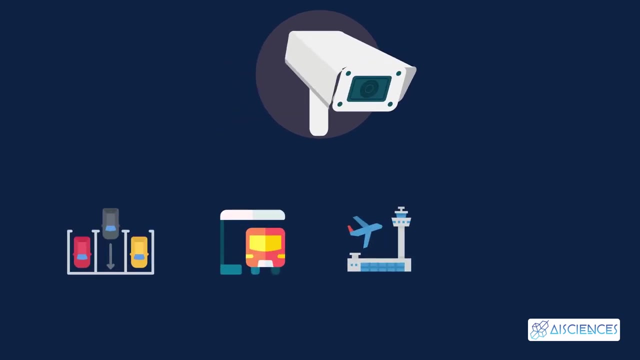 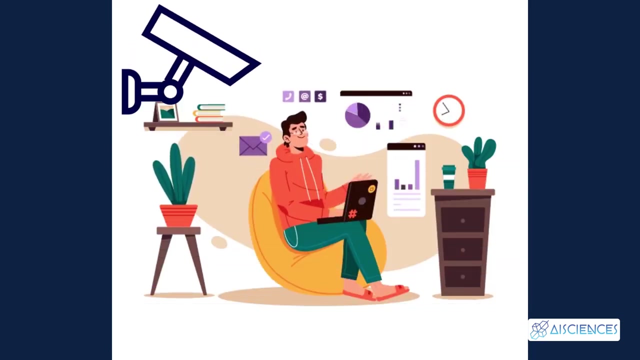 They can also take the right steps in advance. 4. Real-time surveillance: Constant surveillance of public places such as parking lots, bus stations, airports, roads, etc. has become mandatory nowadays. Many private organizations also have 24-hour surveillance cameras to safeguard their 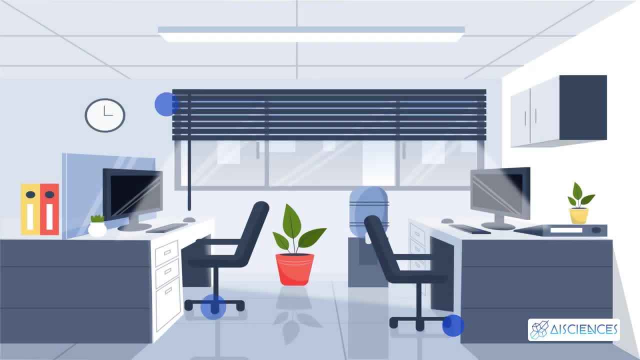 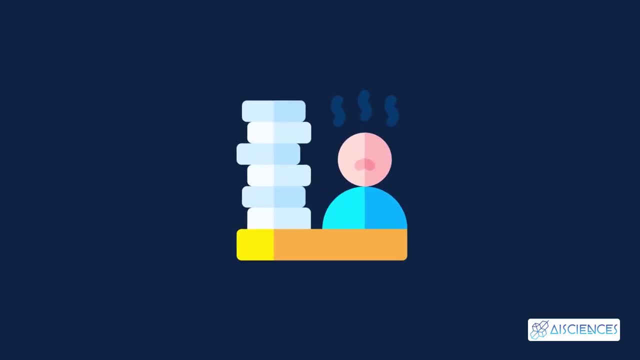 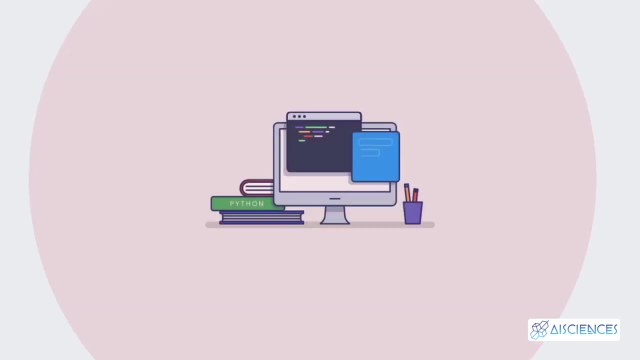 employees and assets. For instance, a single location may have several hundreds of sensors and cameras placed strategically throughout the premises. The data from all these devices would be too complex for humans to monitor, But sophisticated computer vision systems can analyze this data in real-time and send out an alert to the security team as soon as they detect. 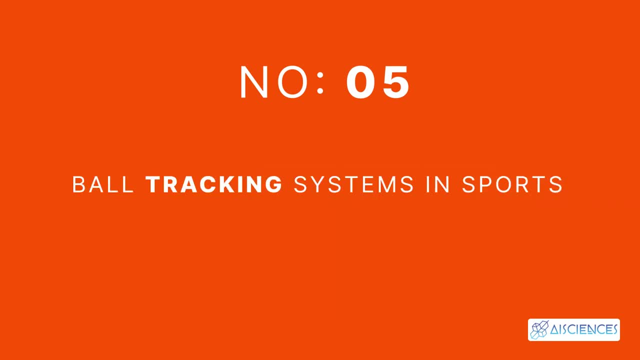 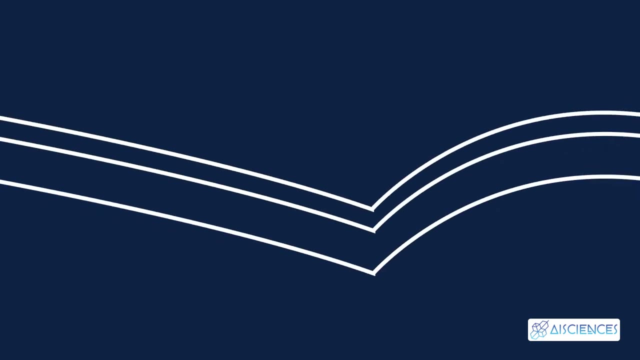 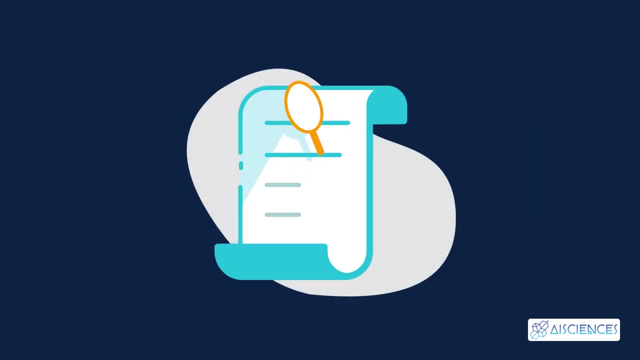 something's amiss. 5. Ball tracking systems in sports. For the last 15 years, precise tennis as well as cricket and badminton ball trajectories are being tracked using computer vision algorithms. Sophisticated systems analyze multiple objects in the image: A three-dimensional trajectory. 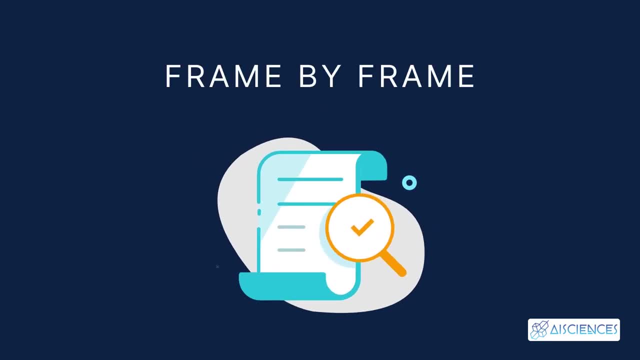 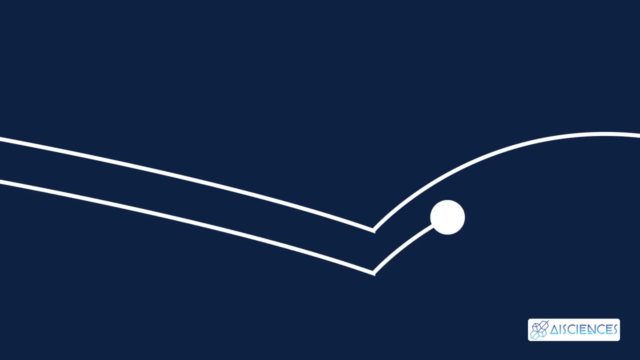 is then built by connecting the pattern of the ball movement frame by frame. Capturing the movement of the ball using multiple camera angles is of utmost importance. The primary purpose is to pinpoint the precise place where the ball landed and determine whether it landed inside or outside the line during the game.